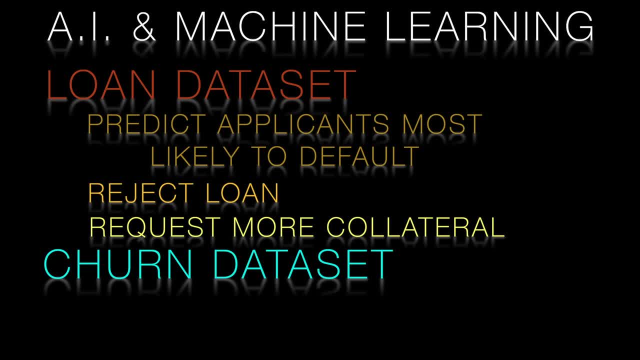 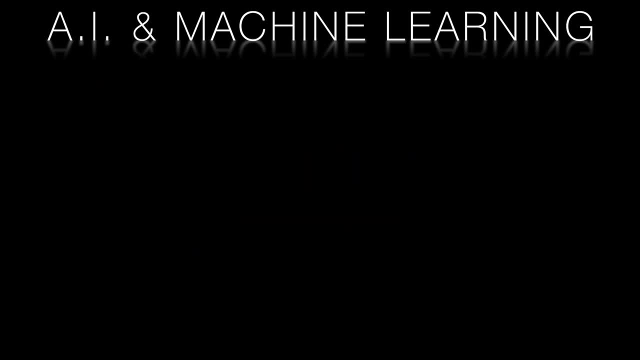 Here, account managers will target these customers with promotions to reduce the likelihood of them losing. Then compare the pay even for an extremely preferred net debt solution, toρού at what bank another borrower should have reached tolearyлив pien. As we will be comparing different AI techniques, it's essential to determine a set of evaluation metrics to assess which type of models perform best on which problems. 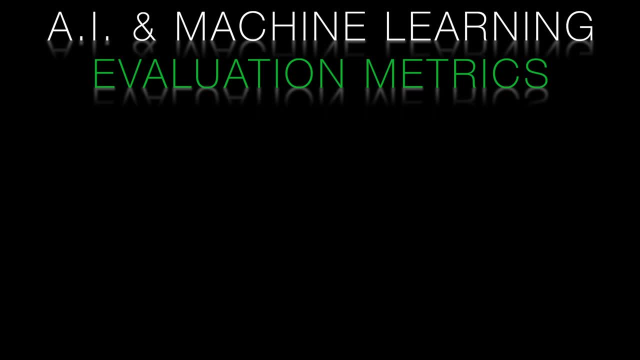 In this video we will discuss several evaluation metrics. We'll start with a counterintuitive assertion that accuracy is a very important function in an association, At least in a non-com hots queued scenario. very poor measure of AI performance. It can be used by unscrupulous developers of AI systems. 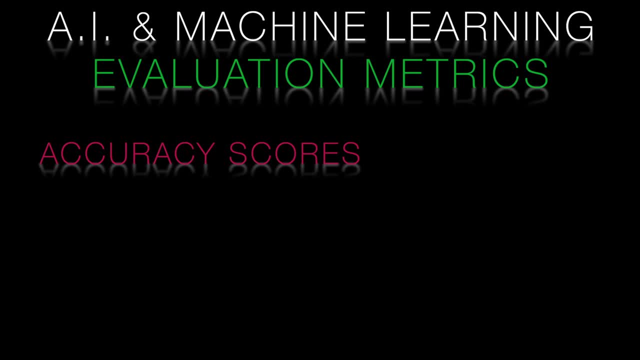 to fool people into believing that their machine learning solutions are better discriminators than they really are. We'll show how to spot this type of fraud so that you won't be misled. To do that, we'll discuss the confusion matrix. This separates out our AI system's correct assertions, The 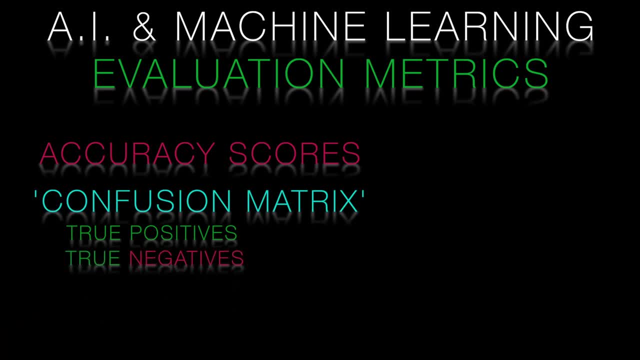 true positives and true negatives Here. the AI is correctly classifying our records. For instance, for a loan default predictor, a correct classification of a defaulting borrower would be a true positive, Whereas a correct classification of a repaying borrower would be a true negative. But 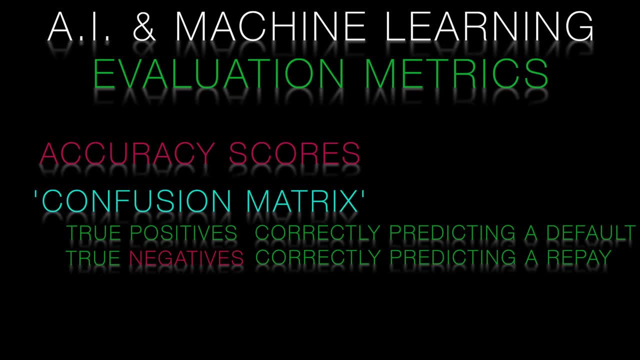 we will also score the wrong data. We will also score the wrong data for the wrongorama, the misclassifications, false positives, where the AI incorrectly asserts that a particular borrower will default, as well as false negatives- Here a classifier predicts that a borrower will. 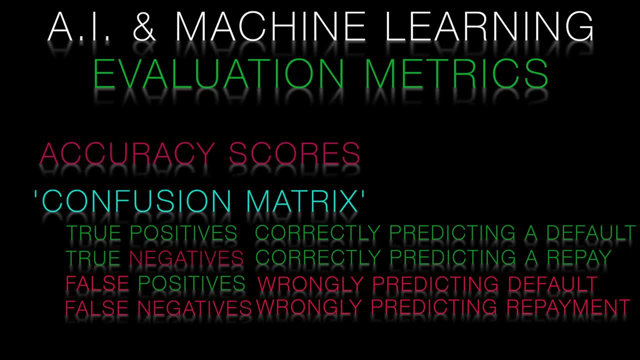 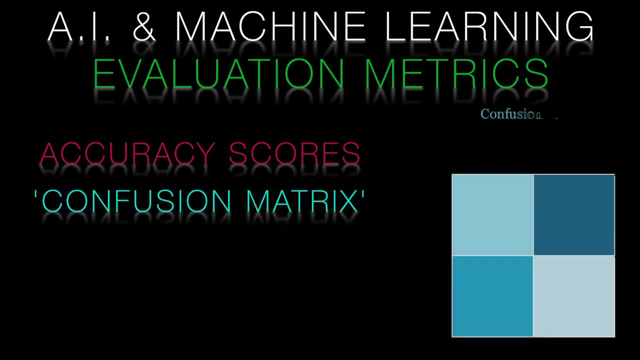 repay when in fact they default. The confusion matrix gives us a great way to visualize the correct and incorrect classifications, to get a better idea of the true performance of a system, rather than relying on accuracy alone. The confusion matrix also allows us to come up with other KPIs for machine learning. These go by the names of precision sensitivity. 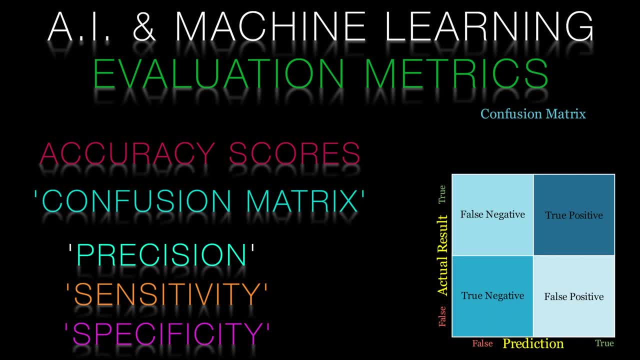 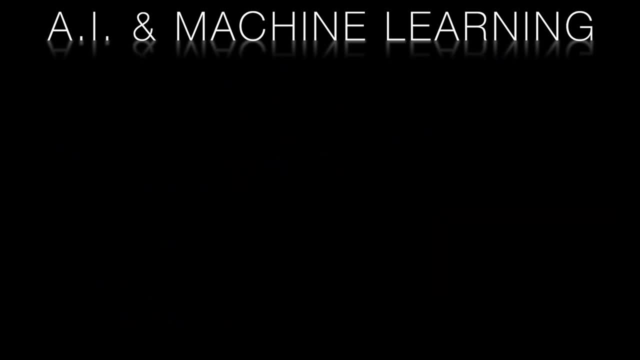 and specificity. We'll describe all of these metrics and how they complement accuracy. in this video We'll see how we can combine all of these metrics to give single scores- an easy way to compare AI solutions. For military history enthusiasts, this will reprise some measures. 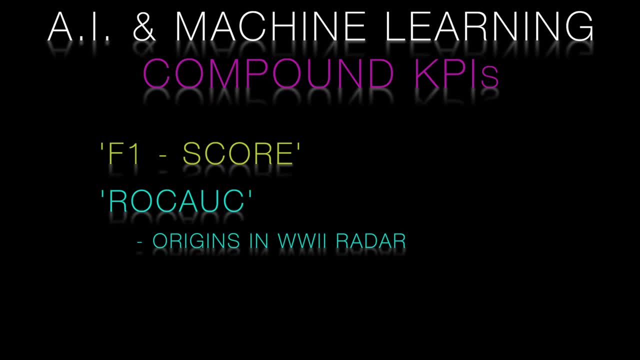 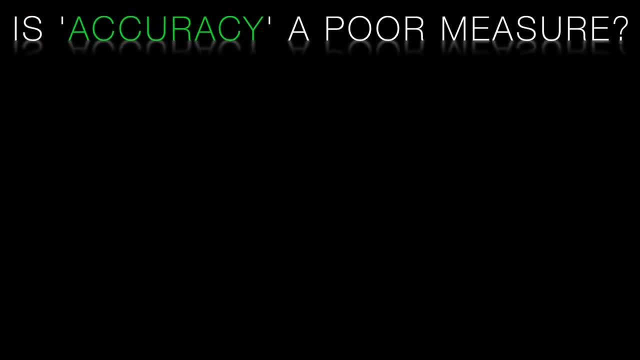 first proposed in the 1940s to analyze radar systems. So let's begin with the perhaps surprising assertion that accuracy is at best a very poor measure of AI performance. At worst, it can be used by bad actors to mislead people into thinking that 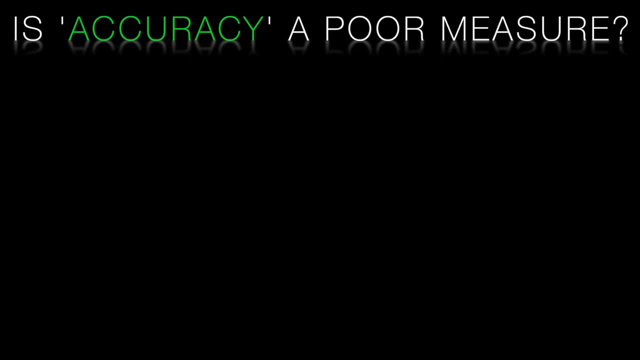 for example, the AI solution is better than it really is. This seemingly benign and innocent equation at first glance might seem harmless and useful: The number of correct predictions divided by the total number of predictions. Accuracy has the advantage that it's very easy to define. This seems simple and neat. What could be wrong with this? As we will see, 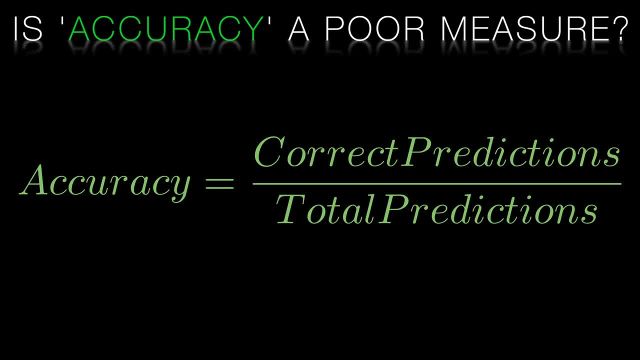 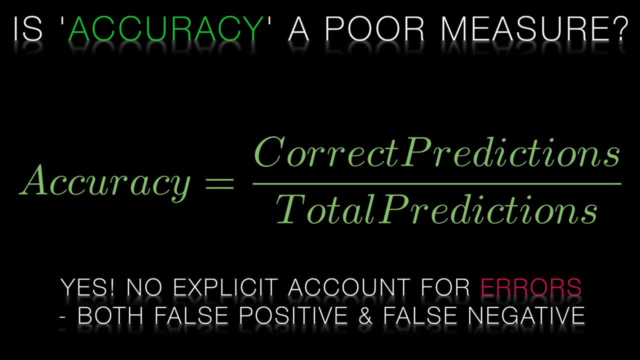 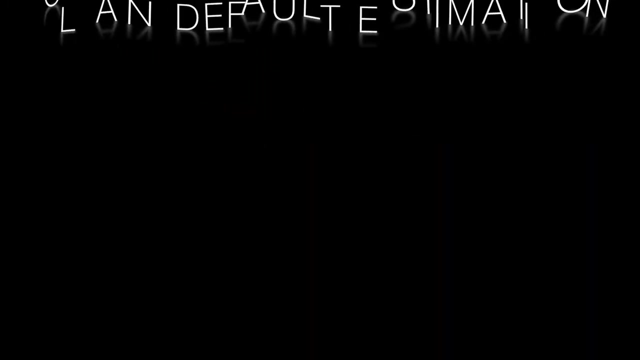 accuracy fails to explicitly take into account false positives and false negatives. In determining a system's performance, it's more important to determine what it got wrong and the type of error- whether false positive or false negative- than what it got right. To illustrate this, 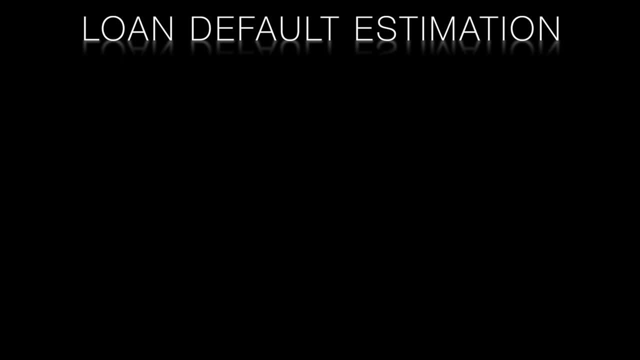 let's look at a very simple loan data set. To keep the illustration simple, we'll just look at two of the inputs Here. we have overdraft utilization on the x-axis and debt to income ratio on the y-axis. We have an output of two classifications as: 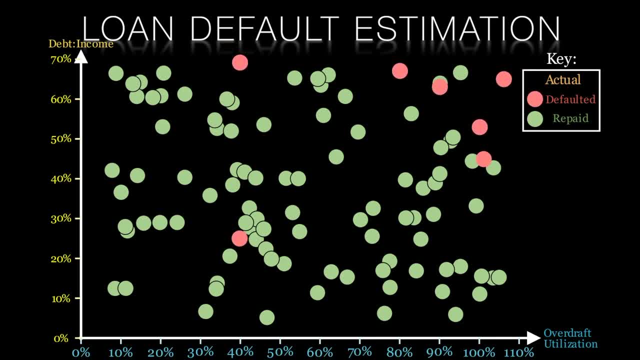 our target whether a borrower defaulted, shown in red, or whether they repaid, shown in green. In this data set, we have seven borrowers who defaulted and ninety-three borrowers who actually repaid. As you can see, the defaulters typically had high overdraft utilization and 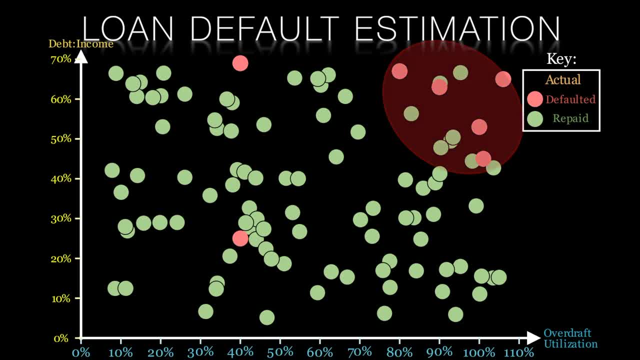 high debt relative to their income. Not particularly surprising. We can use this data set to train an AI model and get it to predict whether a borrower defaults or repays For our predictions. we'll put a circle around each point: red for a predicted. 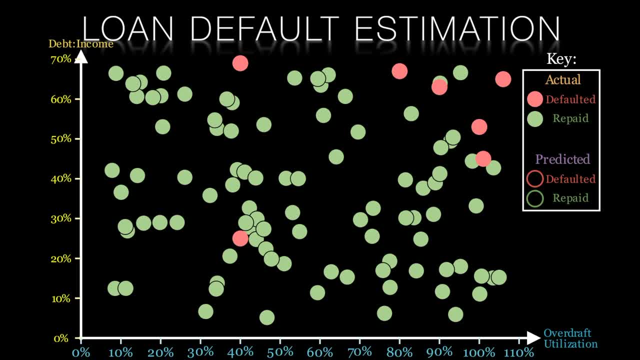 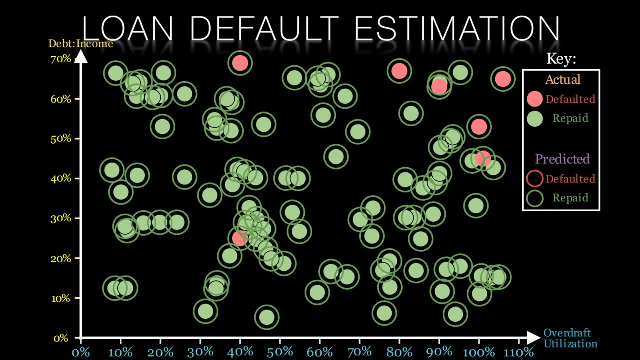 default and green for a prediction of repay. With an unbalanced data set such as this, it's very simple to get an accuracy score of 93%. Just predict that every loanie is going to repay. There is nothing remotely intelligent about this approach. It's merely exploiting the fact. 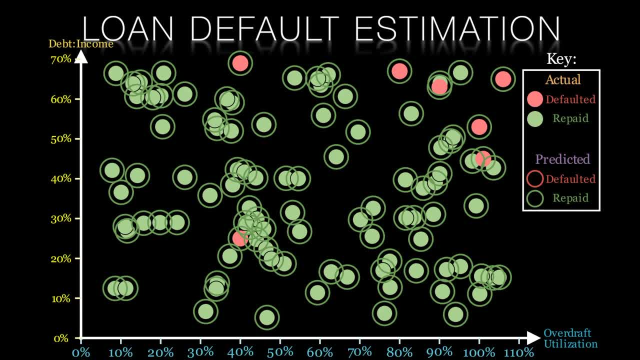 that this is a biased data set, with most of the values belonging to one category. Presenting accuracy like this is fraud and it gives a misleadingly high score. Beware of this. A more plausible AI classifier will get a small number of things wrong, but we'd expect to see a 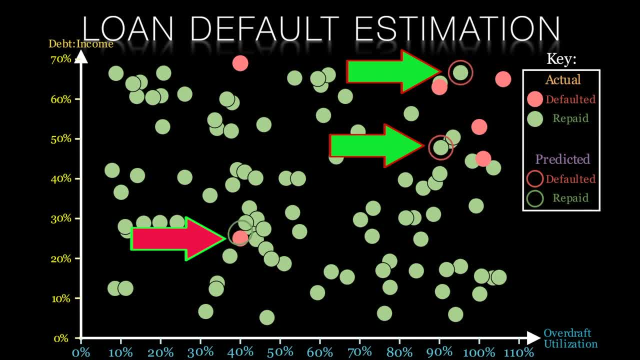 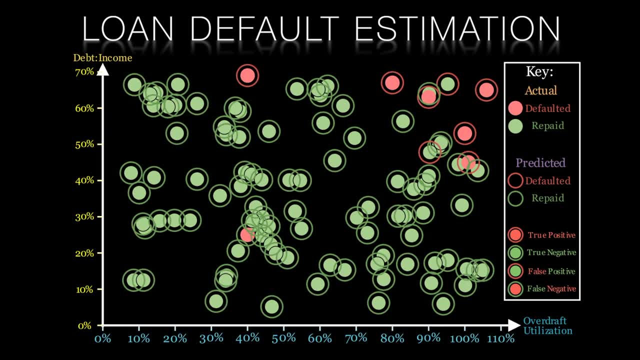 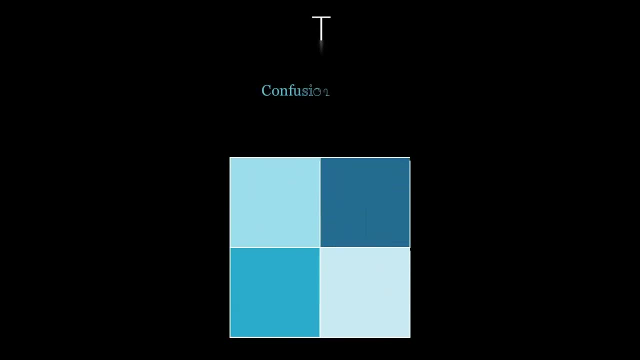 balance of false positives and false negatives. Let's introduce our confusion matrix to see how it can help us better describe our problem. Let's see how it can help us better describe the performance of our systems. We use a a 2 by 2 grid. The rows represent our actual results. 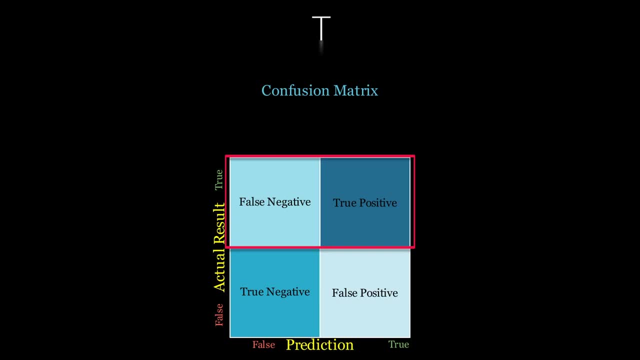 The top row contains all of the actual defaults. In our current lo diezfault example, there are a total of 7 of these. The bottom row contains all the samples where the borrower repaid Again. for our sample dataset, this will total to 93.. This means that all 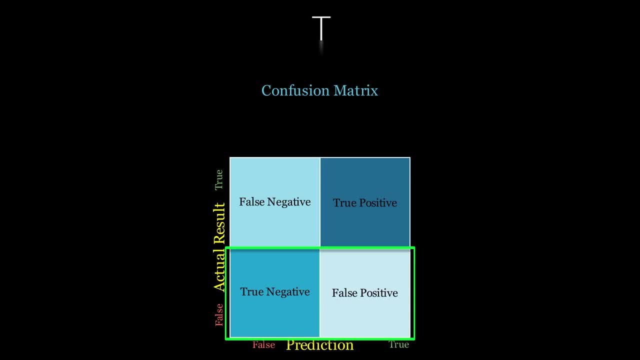 the sample data we sent out are new to the system, which is already valid. Any progress would be guaranteed. I'll take a look at the default system list again. The checking page shows the. This means that our correct classifications will lie on this diagonal. 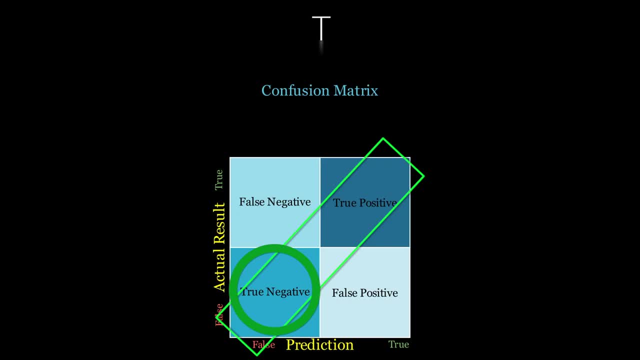 Bottom left contains the correctly classified repayers and top right correctly classified defaulters. Our incorrect classifications will lie on this diagonal. Top left is where the AI believed a sample would repay when in actual fact they defaulted. Bottom right are all of our classifications where the opposite occurred. 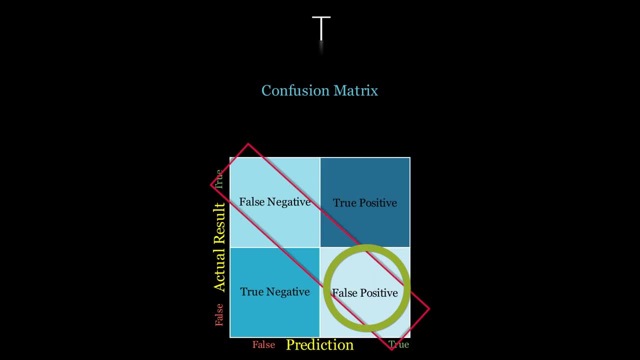 The AI asserted that the sample would default when actually it repaid. In this example, we could also add some qualitative attributes to these classifications. In the top left, our model was complacent, approving a loan application that actually defaulted. On the bottom right, it was fearful, denying a loan applicant that actually went on to repay. 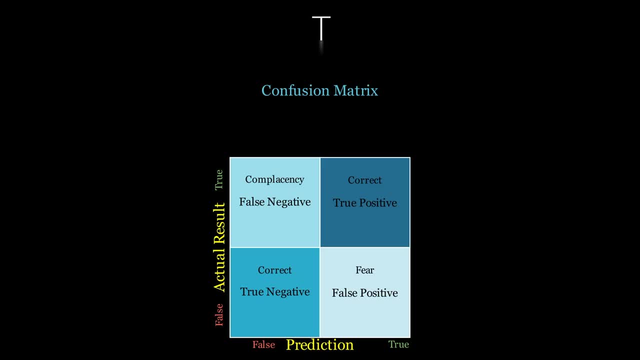 We can use the confusion matrix to quantify. We can use the confusion matrix to quantify key ratios and describe the performance of our model. We have a much larger sample of borrowers repaying than defaulting. For our smaller defaulting sample, we can look at the number of correctly predicted defaults relative to all defaults. 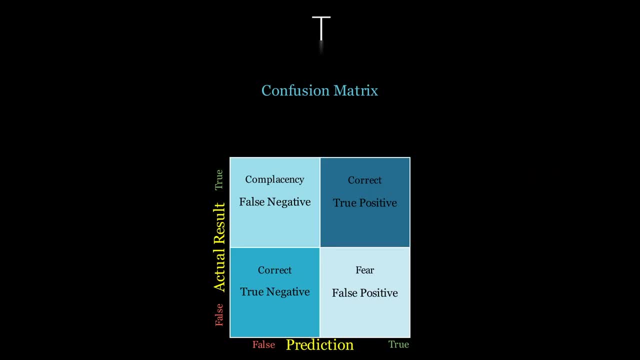 This ratio is called the sensitivity. Likewise, we can look at the number of correctly predicted repayers relative to all the repayers, And this is called the specificity, And this is called the specificity. Our columns in the confusion matrix show us our predictions. 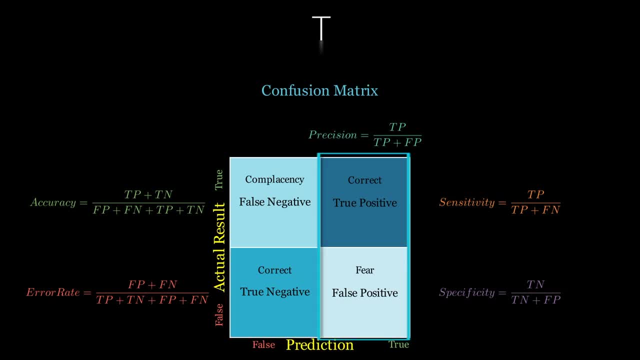 We can derive the model's precision and this is the ratio of the correct positive predictions relative to all positive predictions. Use of all these metrics helps us to put the accuracy metric in better context. It's not that we shouldn't use accuracy, but we should use the accuracy in context of the other metrics in the model. 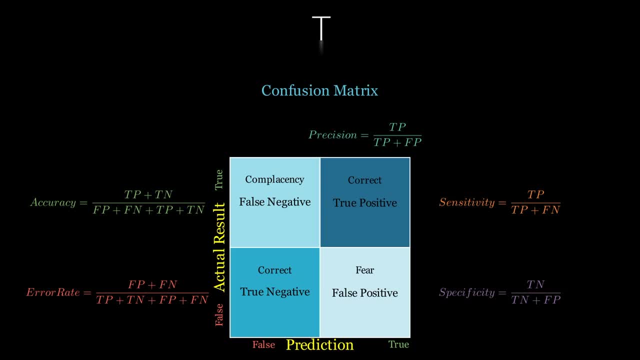 and KPIs derived from the confusion matrix. Let's use an example to further illustrate this. If we start with our dubious classifier that simply classified everything as a non-defaulter, then we have the following confusion matrix: Our accuracy is an impressive 93%, but as soon as we 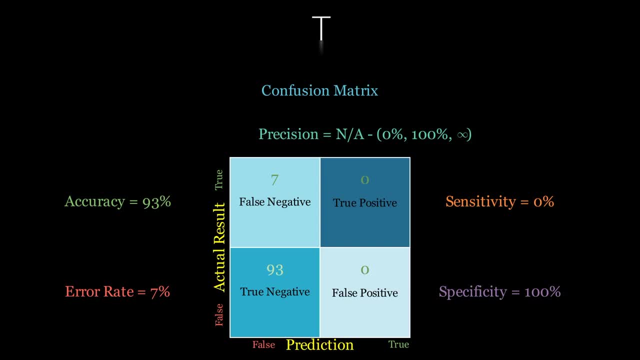 start looking at our precision, which is indeterminate as we have a divide by zero, and our sensitivity, which is zero percent, then the shine somewhat falls off our accuracy number If we instead look at a more plausible example that correctly predicts five of the seven defaulted. 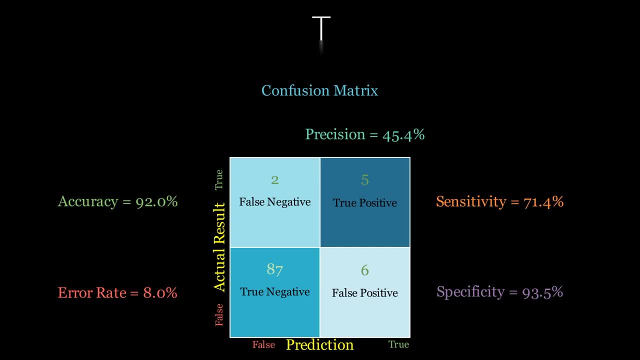 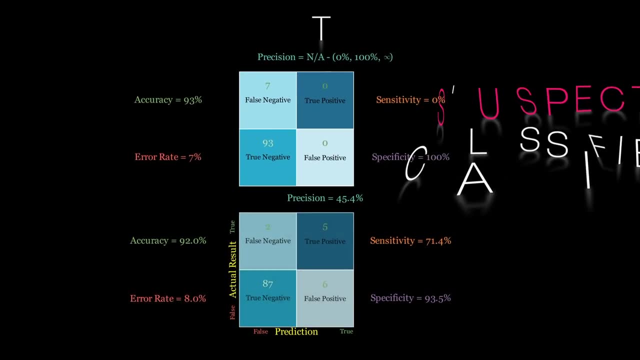 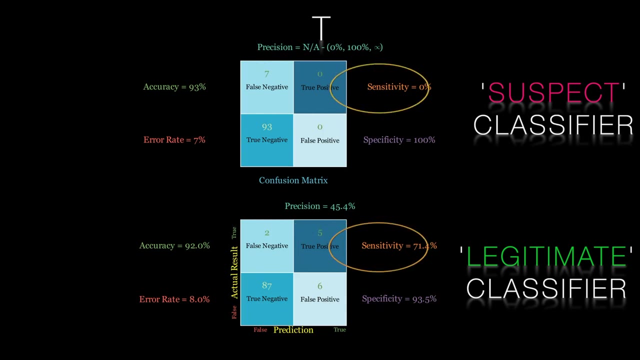 loans, as well as 87 of the 93 repaid loans, we get this picture. Note that the accuracy is not as high- it's only 92%- but this is bolstered. This is bolstered by a sensitivity score of 71.4%, as five of our total of seven defaulted. 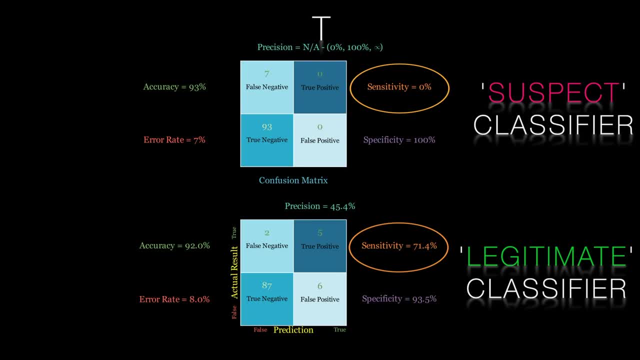 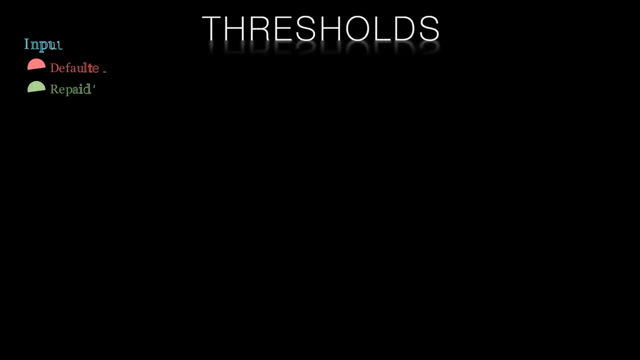 loans have been correctly predicted, as well as a precision of 45.4%, reflecting the fact that five of our 11 predicted defaults were correct. We can also use our confusion matrix to help calibrate our model to achieve optimum results. Our test data's target record. 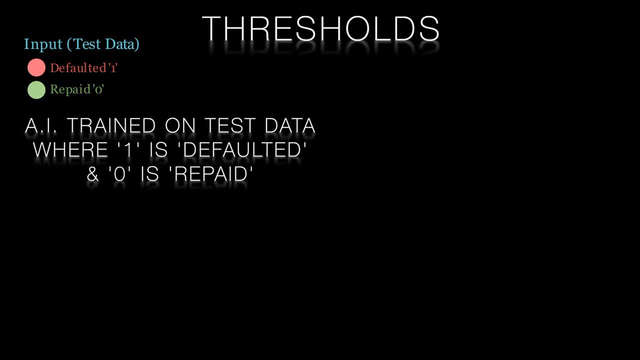 is the defaulted flag. This will be one if the borrower defaulted and zero if this borrower repaid. The output of our trained model will never exactly be one or zero. it will take on a continuous range of values reflecting the likelihood of default. The higher the number. 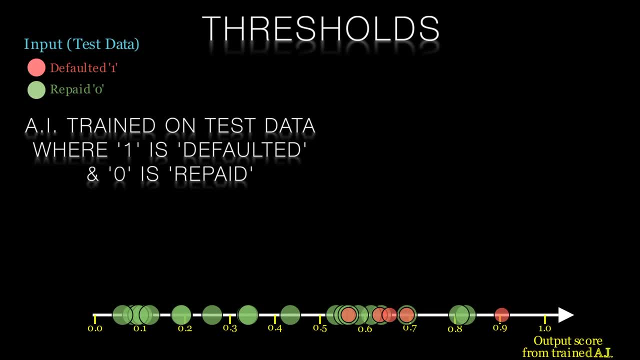 output by a classifier, the more likely a default. So where should we set our threshold to separate our probability of default? We should set our threshold to a threshold of predictions into defaulters and repayers. An obvious, maybe intuitive, answer is 0.5.. 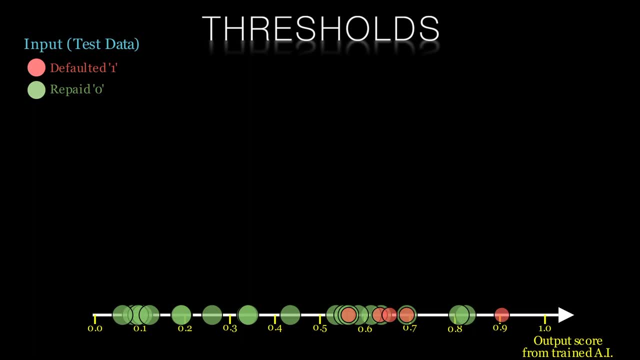 Anything above 0.5 will be classified as a defaulter and below 0.5, a borrower, who will repay? While maybe not a bad start, it's unlikely to be the optimum threshold value. Let's see why. Here we see 25 examples used to test our 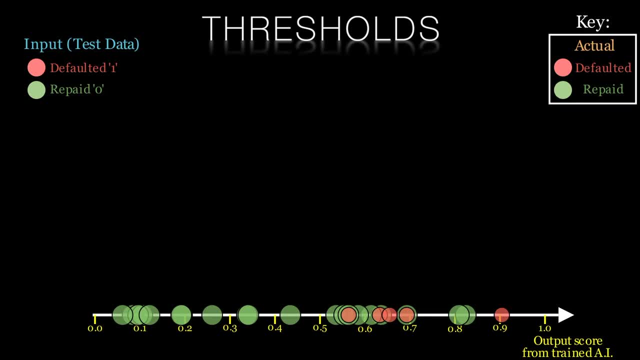 AI system. The borrowers that actually defaulted are shown in red and the repayers are shown in green. The position of the coloured dot on the X axis represents the score assigned by the AI system to this borrower. The higher the score, the more confident the AI system. 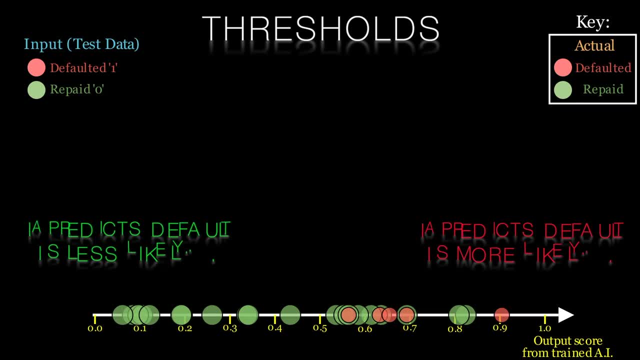 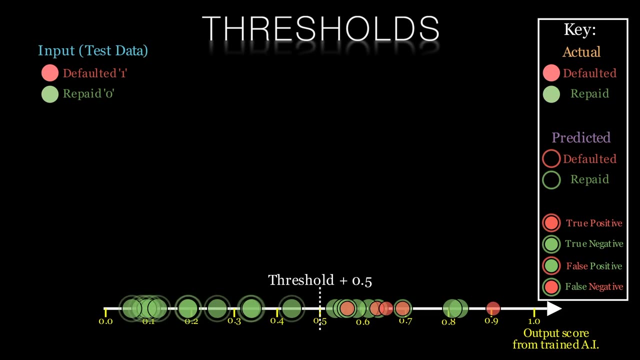 is that the borrower will default and that the loan should not be approved. We are interested in the AI's predictions. These can be assigned to the four quadrants of our confusion matrix. If we set our threshold to 0.5, then every score below 0.5 will be predicted to repay. 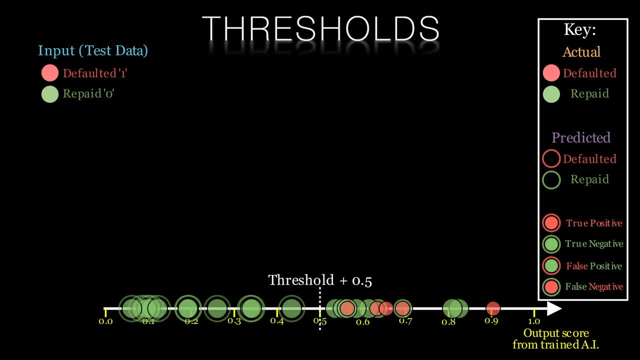 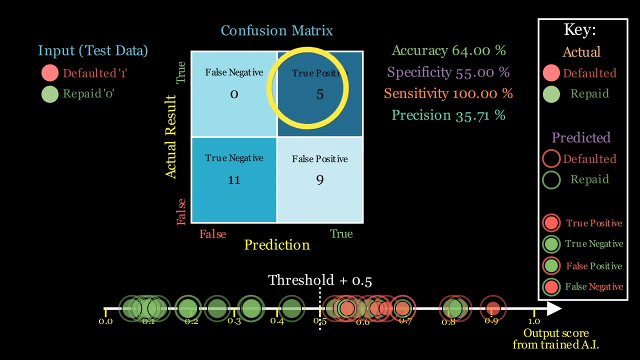 and we'll circle these in green And every score above 0.5 will be predicted to default circled in red. This will result in the following confusion matrix: We have no false negatives at all. We correctly find all the defaulters, our true positives. Our model is very sensitive. 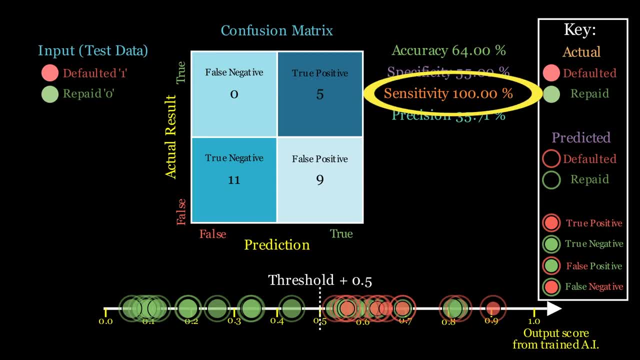 to finding all the defaulting loans and it gets a great sensitivity score to reflect this. However, we incorrectly assign 9 borrowers to the defaulters category And with 9 false positives, both our precision and specificity scores suffer. Our accuracy is 64%. 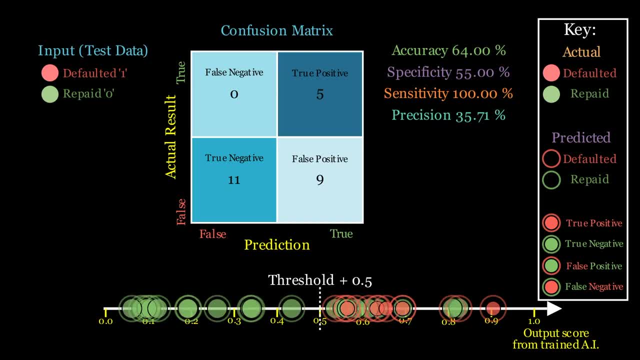 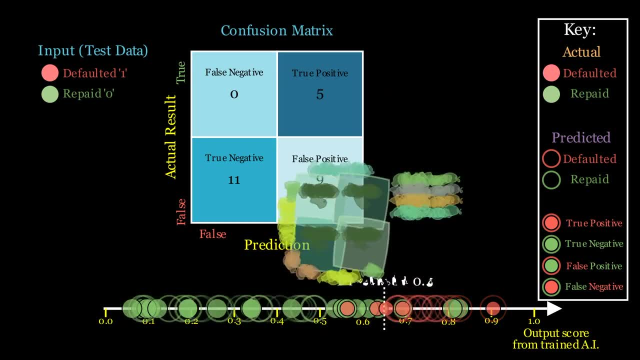 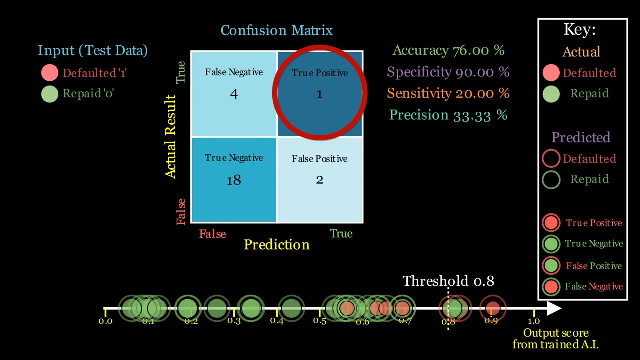 So is 0.5 the best threshold? Let's push our threshold up to 0.8.. Here we only correctly assign one defaulter. If we used this threshold on this model for loan approval, then we would make 4 loans to borrowers who would not pay back. Perhaps this is not ideal. Note again: 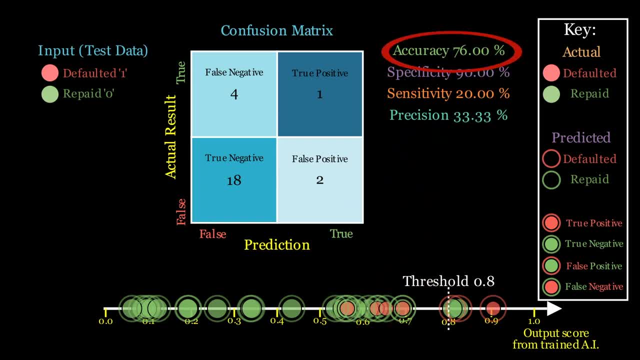 here that our accuracy score has increased from 64%. About 50% of borrowers are still 64% to 75%. Yet this doesn't seem as good a model as having the threshold at 0.5.. So if we lower the threshold to 0.545, we get a more balanced result At this threshold. 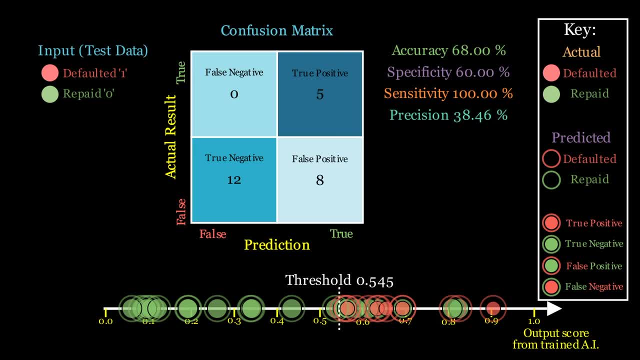 we have no false negatives. We aren't making loans to borrowers that will default, And here we have only 8 false positives. This means better precision and specificity scores than when the threshold is at 0.5.. A great compromise for this model, would seem. 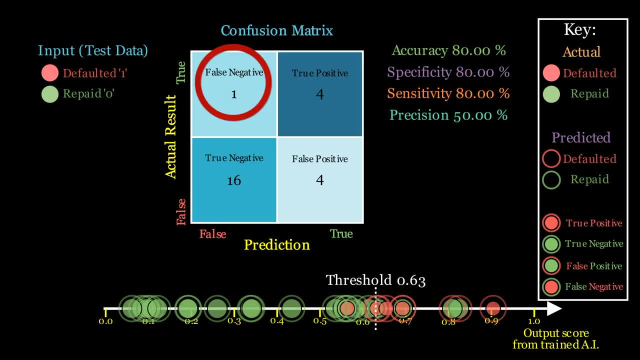 to be a threshold of 0.63.. While we misclassify one defaulter, we only misclassify 4 repayers. This is reflected with high scores across all of our KPIs, So is 0.63 the best threshold for this model. 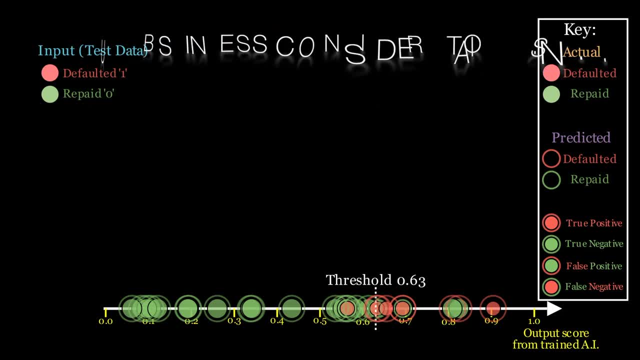 Well, it depends. There are business factors to consider. If these loans are fully collateralised with high quality assets that can be assigned to the lender in the event of a default. if loan arrangement fees are high and interest rates are high, then you might tolerate an even higher threshold. 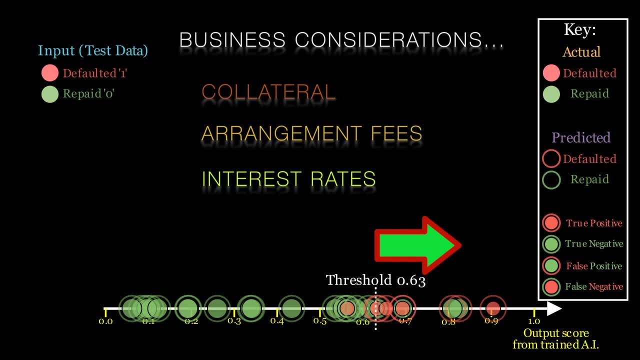 For sure we will approve loans that will default, but our downside risk is mitigated with the collateral and we are compensated for our lending risk with a quality revenue stream, On the other hand, with low interest payments, zero loan arrangement fees and uncollateralised loans. 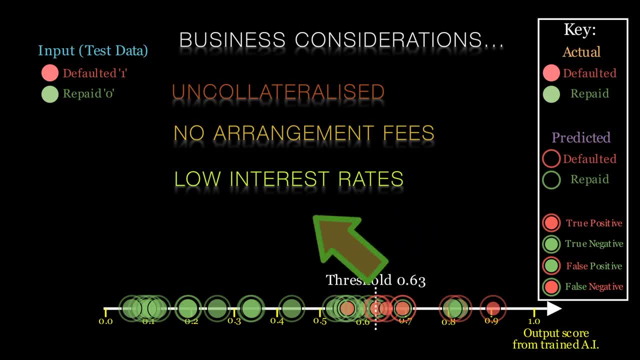 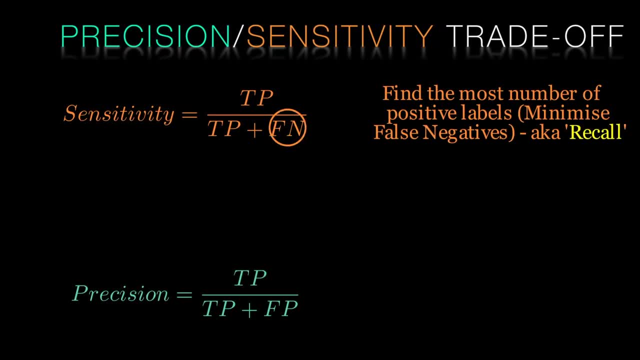 then we would be wise to set our threshold lower. This boils down to a precision approach. If you recall how the ratios are constructed, you can either have a high precision or a high sensitivity, but not both, Given your business case, that is to say, your collateral terms, loan arrangement fees, interest payments. 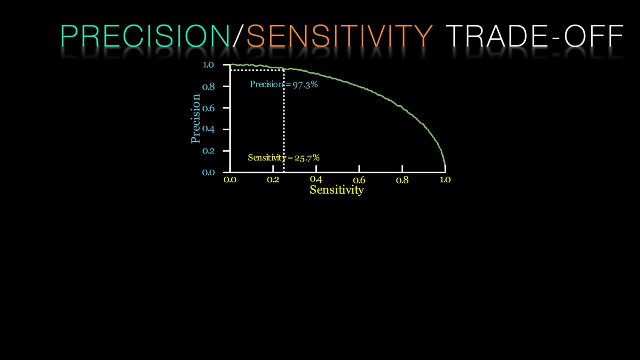 you can use the precision sensitivity curve to determine your optimum threshold. You can also use these metrics to compare alternative models. As you want to maximise both precision and sensitivity, then you would always favour the model with the green curve over a model with the red curve. 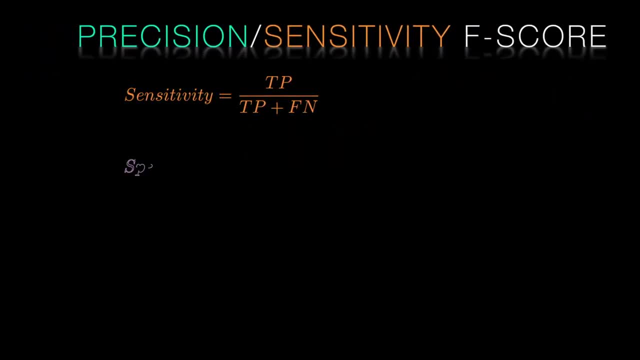 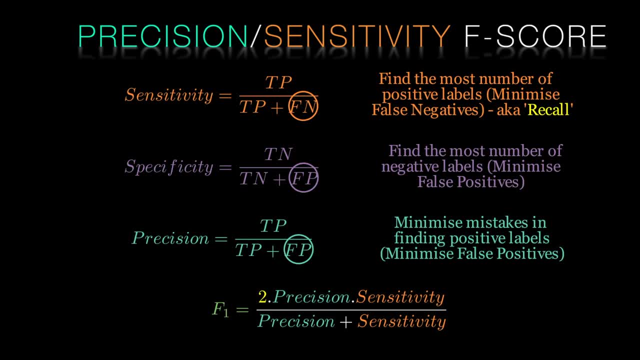 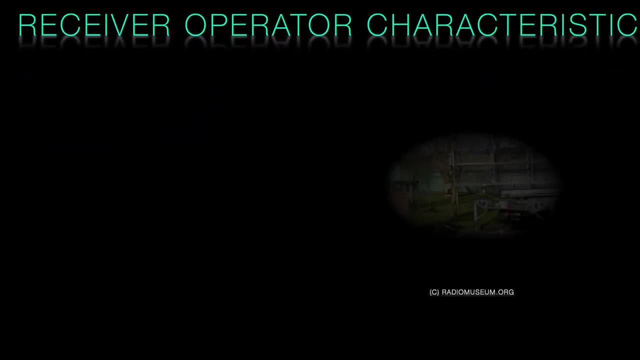 actually it's the harmonic mean, which is twice the product divided by the sum of the precision and sensitivity. The F1 score is a very useful heuristic to compare different models. Perhaps the most widely used measure for comparing AI models has its origins in the early uses of radar. 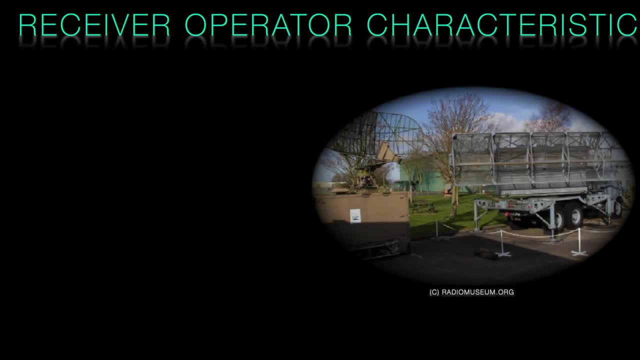 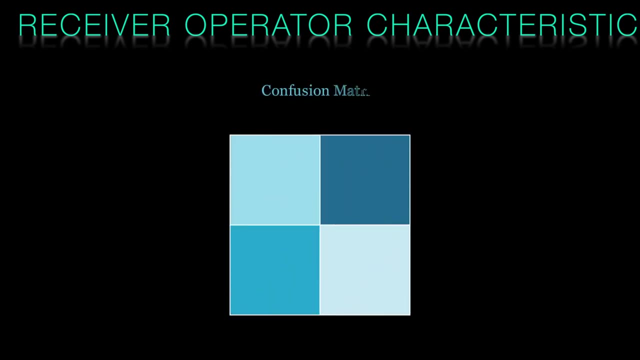 in the Second World War At its heart. a radar is a classifier used to detect enemy aircraft or ships. True positives are an incoming sortie of enemy aircraft. True negatives are when the sky is clear. False positives might be brought about by a flock of seabirds. False negatives are a failure to. 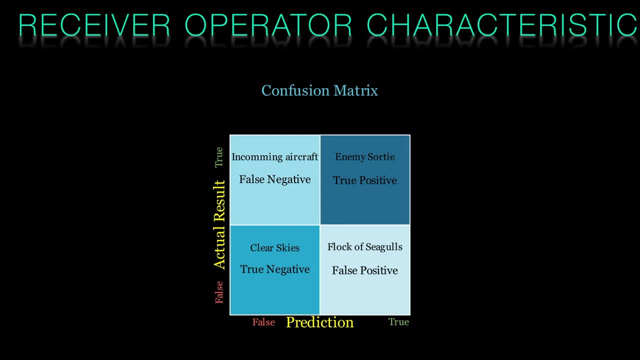 detect an incoming aircraft, Air Command. Air Command and air command were needed to set their thresholds correctly and to do so used ROC curves. ROC stands for receiver-operator characteristic. The setting of the threshold involved the tuning of the radar receiver by the operator. The classic ROC curve plots the true positive rate versus the 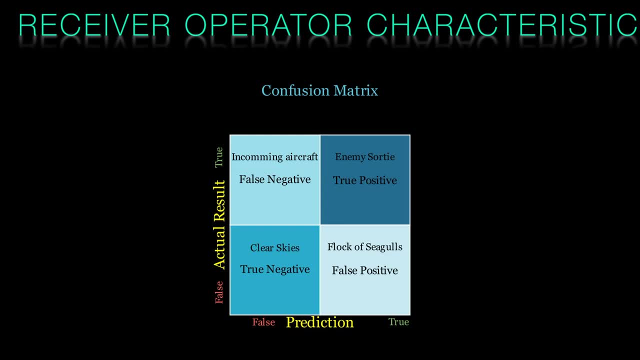 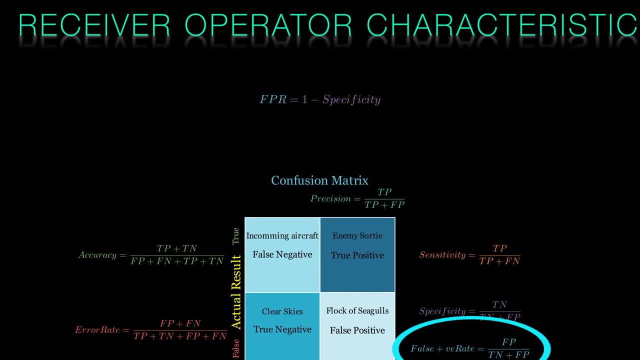 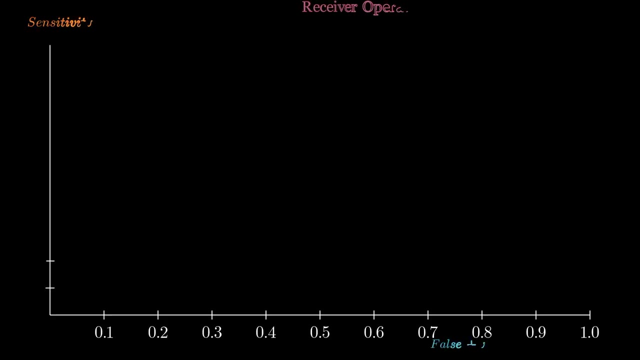 false positive rate. The true positive rate is what we've been calling sensitivity, And the false positive positive rate is 1 minus the specificity. What you want is a threshold that gives you a high true positive rate whilst at the same time giving you a low false positive rate, By plotting this: 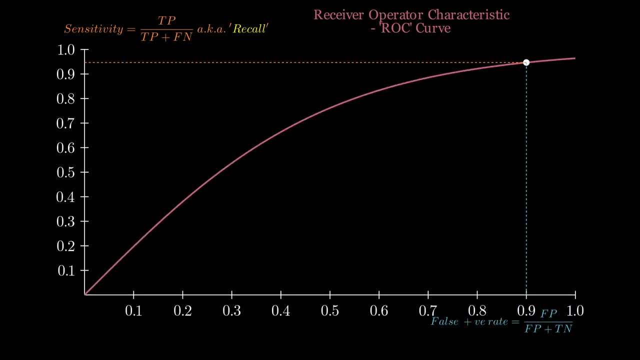 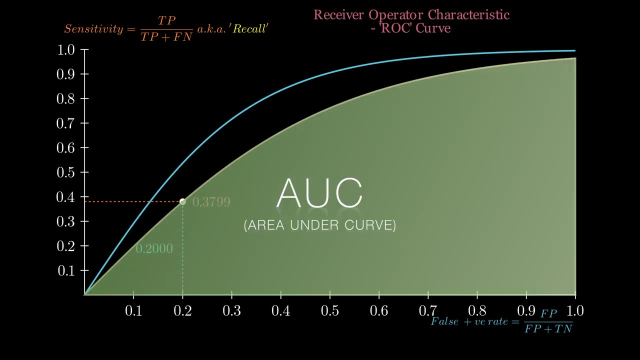 curve. you can choose a threshold value to achieve this. Just as important is, you can use these curves to compare different models. The area under the ROC curve, usually abbreviated to ROC AUC, can be found for each model In the example on the screen: the model with the blue ROC curve. 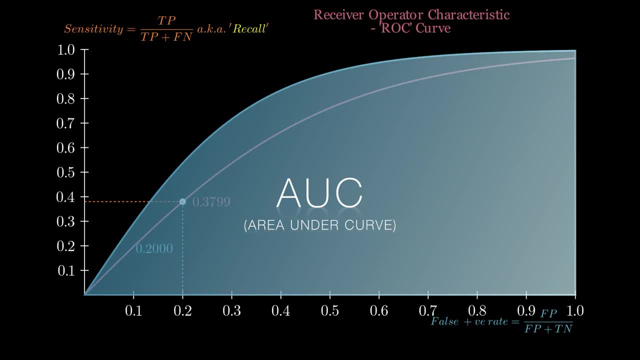 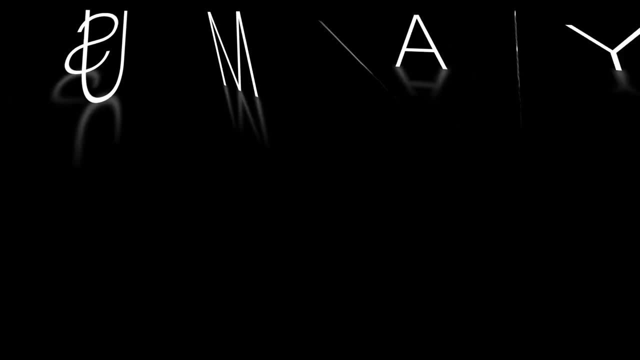 is superior to the one with the red ROC curve, while the model with the yellow curve is the best of all. This is Richard Walker from Lucidate. Many thanks for watching this first video on machine learning. This episode we've looked at KPIs for our AI and machine learning models. We've seen how accuracy